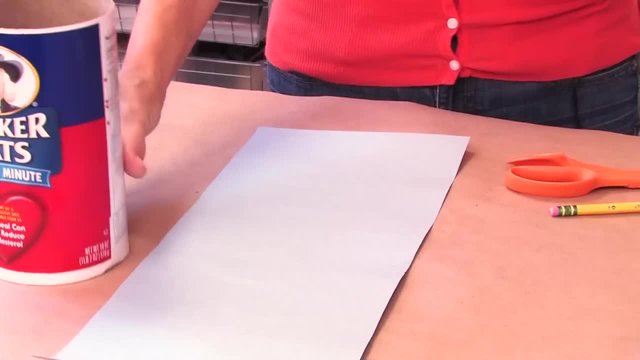 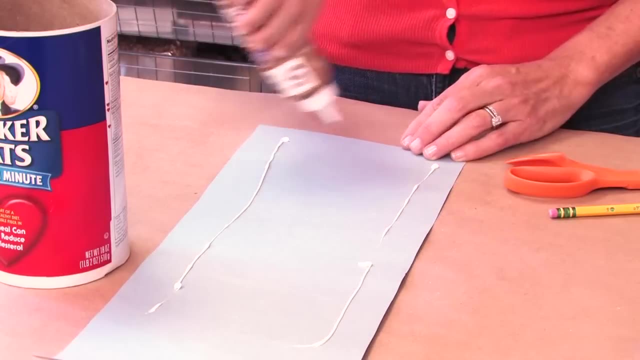 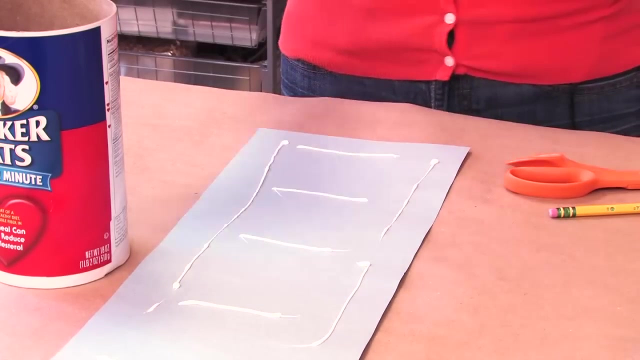 use double-sided tape if you'd like. whatever you have, that's easy. I have some tacky glue, so I'm just going to use that. We're just going to glue our strip of construction paper right onto our roll Tom tom drum, and we can make lots of noise this Thanksgiving holiday. Here we go Just. 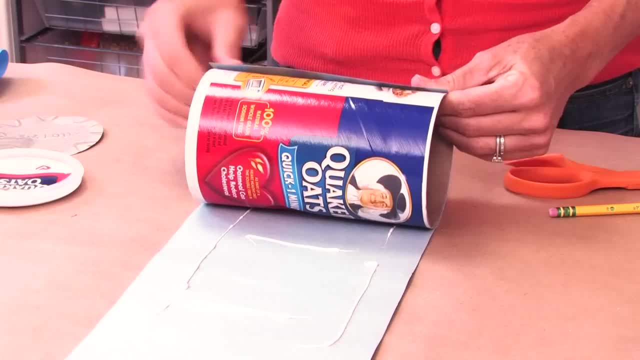 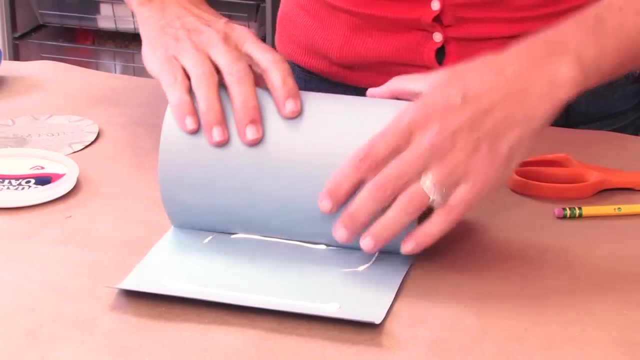 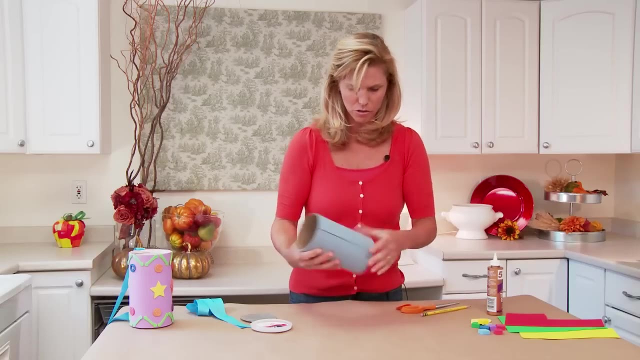 kind of roll it right around. This is a great craft for the kids because it's so easy and they love it because you know they'll be making noise and they love to make noise. So just keep it straight and even if it's a little crooked, a little off, that's fine, We can. 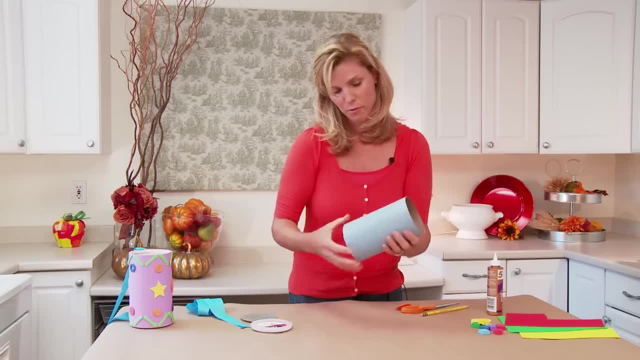 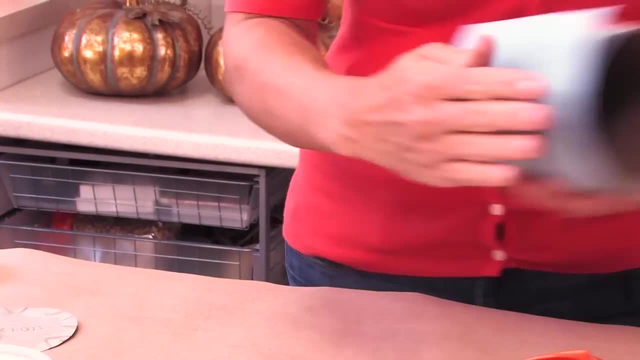 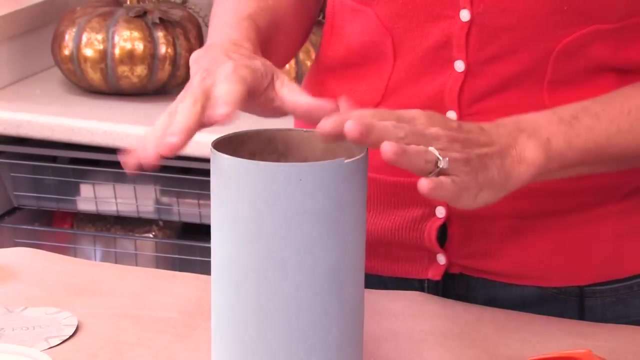 trim. you know, the perfection is in the imperfection. that's what I say. So we just need a little bit more glue here, just to pop down the ends, just like that. Okay, Now to decorate we. 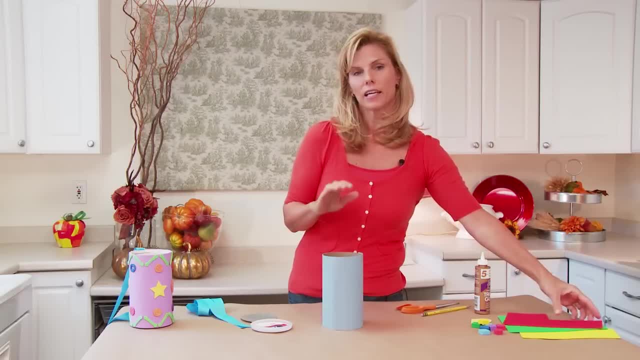 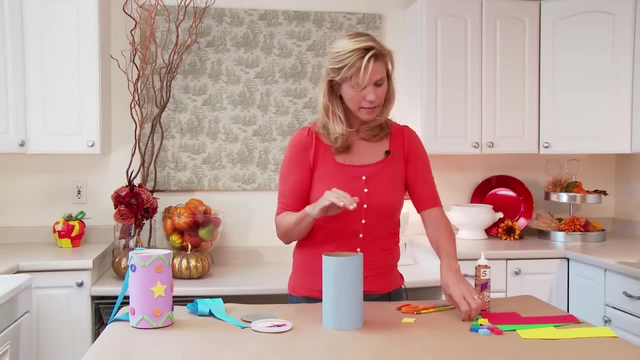 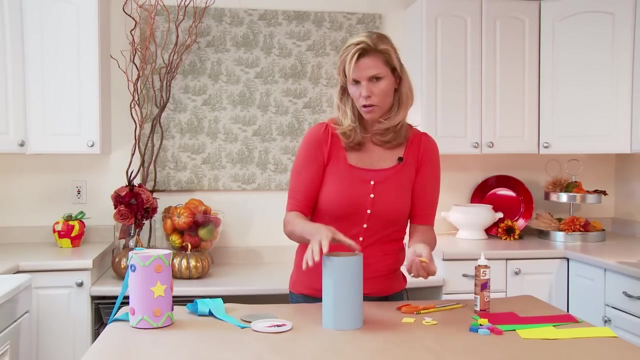 can use all kinds of different shapes that they can cut out of construction paper. or, you know, I have a happen to have a huge collection of the foamy shapes and letters. I'm just using a bunch of those and just so easy, I mean look at this and then they go around and 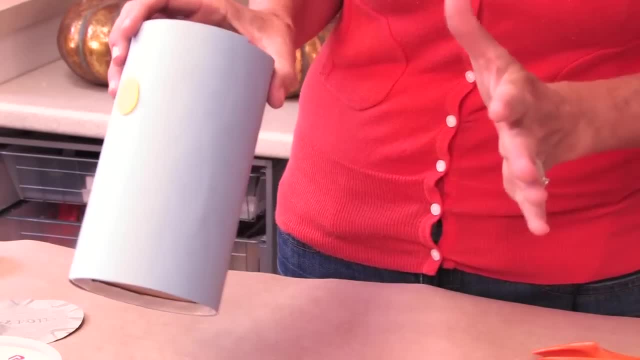 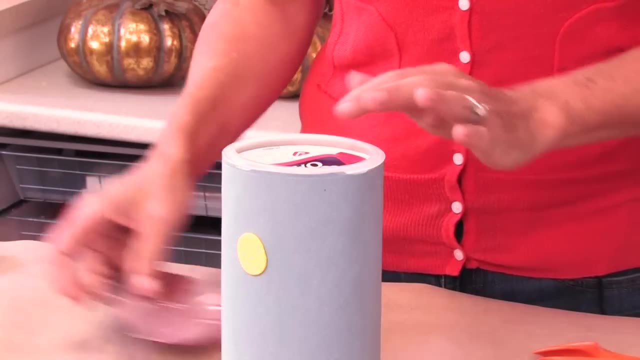 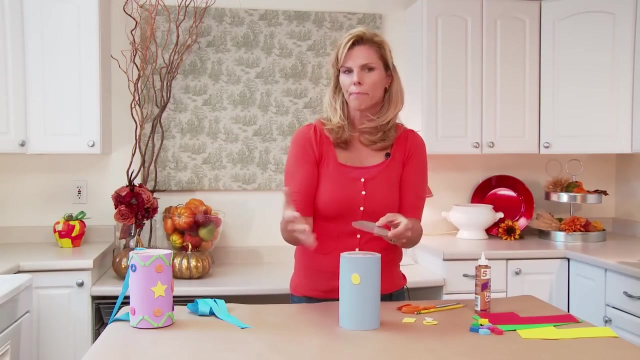 they create their own little pattern. I mean, how easy is that? can you stand it? it's so great. then put the top back on, and what I do to create a little place where they can tom-tom is you know those little aluminum foil dishes that you have all the time. I know you have some. 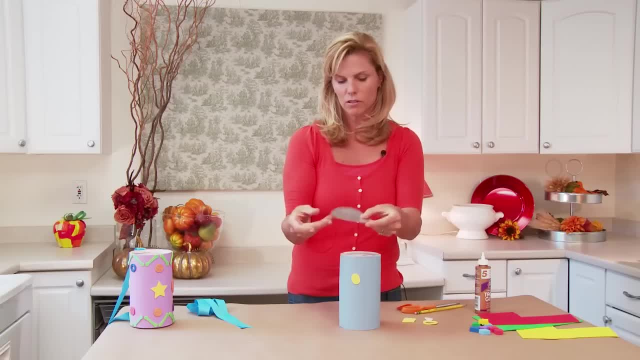 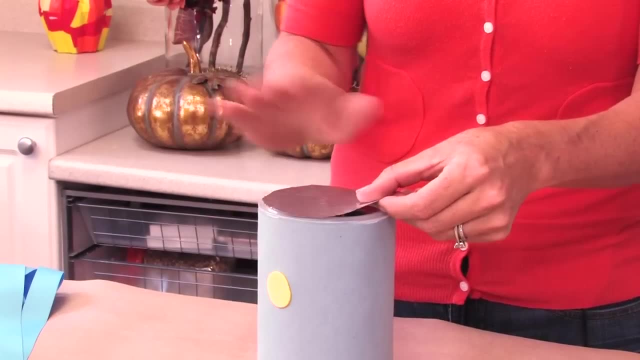 so you just grab one or two of those and cut out circles. it just kind of makes it decorative and it also makes a really great noise. so you just cut it out and you put it right on the top and when they go to tom-tom it just kind of makes gives a little extra. 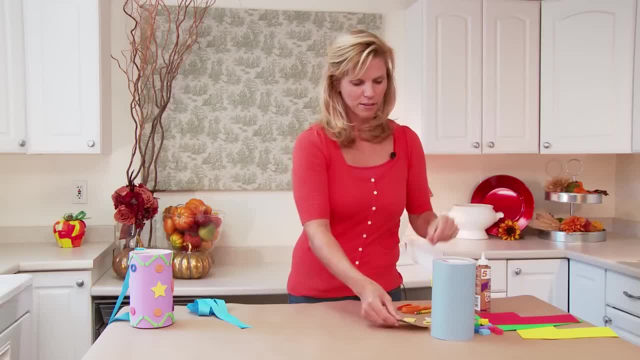 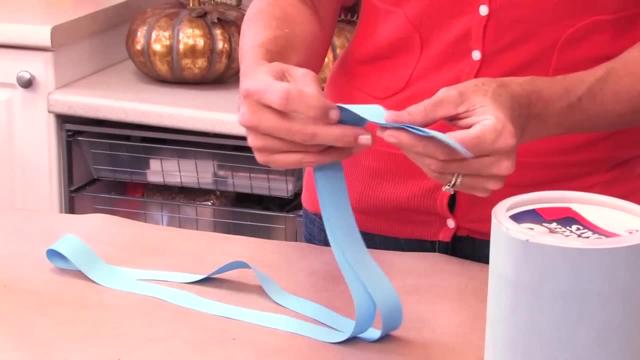 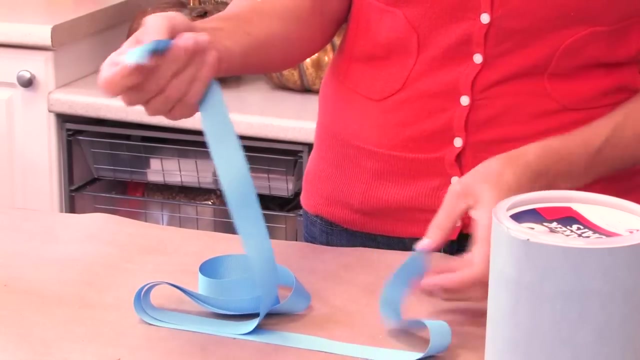 noise for their little drum. now, to finish off, what you're going to need is a ribbon. this is about. this is about 36 inches. you can use any kind of ribbon you have and they house. I happen to have this blue grosgrain, which is perfect for the blue drum. And what?